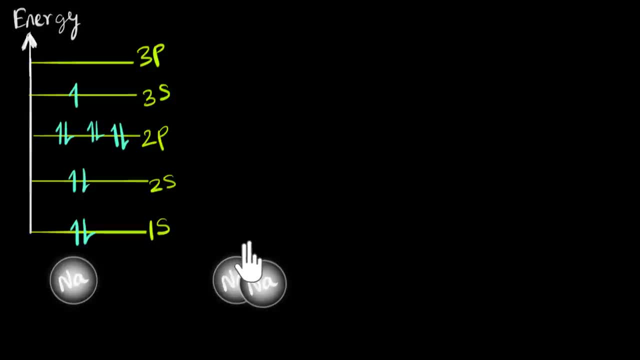 our molecular orbital will end up having two energy levels. So if we are looking at 1s, let me just draw that. So if you redraw the energy level, but now not for the atom, for this entire molecule, then the 1s of this and 1s of this combine and form. 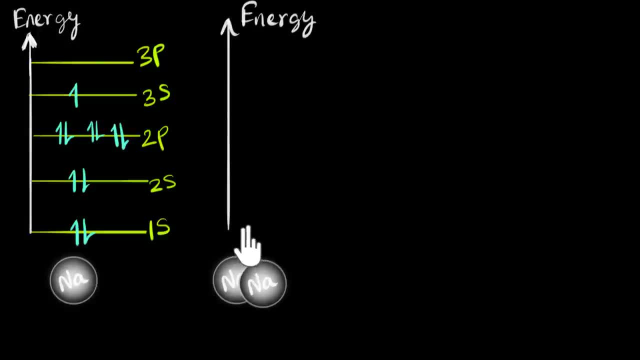 a new 1s molecule. So that's the molecular orbital, And that molecular orbital itself has two energy levels, Two energy levels. These two energy levels belong to 1s molecular orbital. We usually call them as 1s and 1s star. 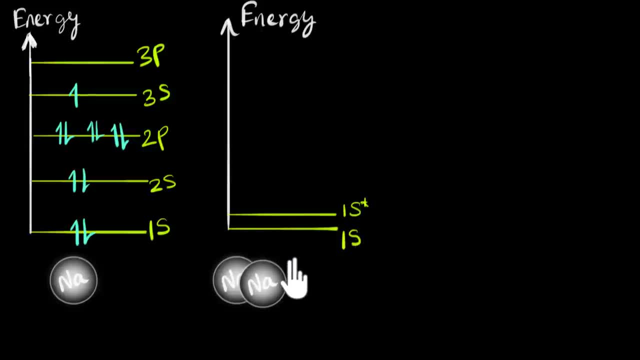 And again, this is something that you may have already learned in chemistry, molecular orbital theory, This lower energy orbital is called as the bonding orbital and the higher energy orbital is called as the anti-bonding orbital. And again, if you need more clarity, 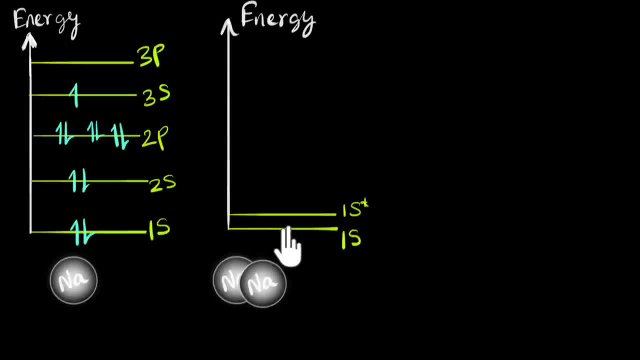 it would be great to go and watch those videos in chemistry, But guess what? We don't need things so rigorously over here. All we need to understand is that the two atomic orbitals combine and become one molecular orbital, and they end up having two energy levels. 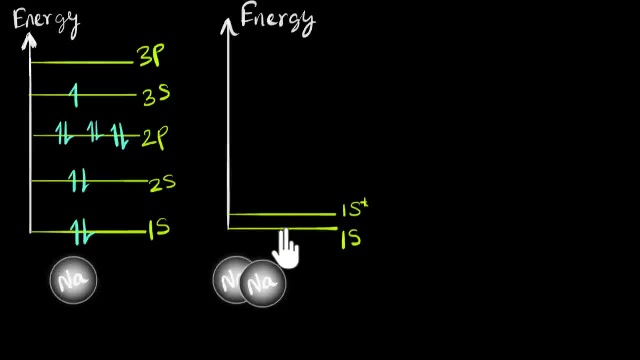 And the way I like to think about this is: I just like to think of this as so conveniently solving Pauli's exclusion principle, Because now the two electrons from this sodium can fill up this level of the molecular orbital, and the two electrons of this sodium can fill up this. 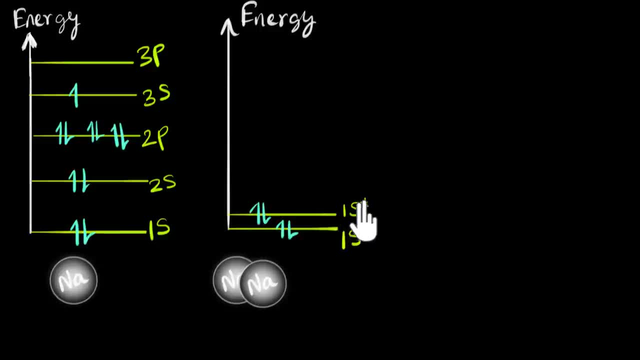 This molecular orbital energy level of the orbital And we are fine. Pauli is now happy because now these two electrons are no longer identical And the same thing is going to happen to our 2s orbitals: They're also going to overlap. 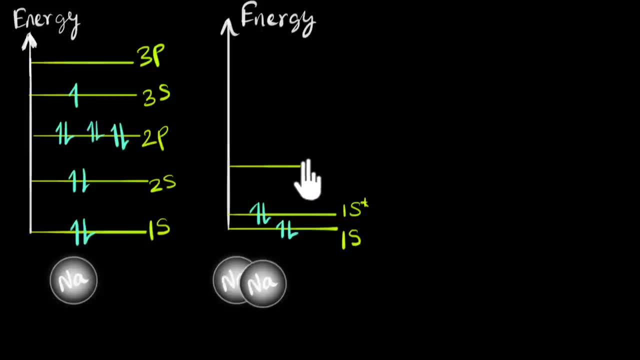 and now you'll have a 2s molecular orbital, which will also have two energy levels. And guess what? We don't have to remember this star stuff. I'm just gonna call this as 1s molecular, 2s molecular, And the same thing is going to happen over here as well. 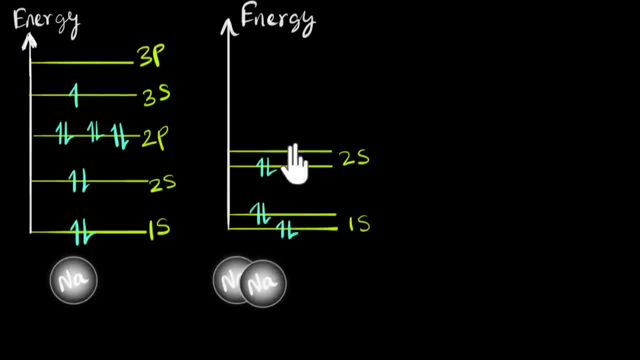 Two electrons from this atom maybe can occupy the lower ones, and the two- is electrons of the other, can occupy the higher ones, and so on and so forth. and now notice, all electrons have different energy levels. so poly is fine now. and so now, what do you think is going to happen if we add a third sodium atom to 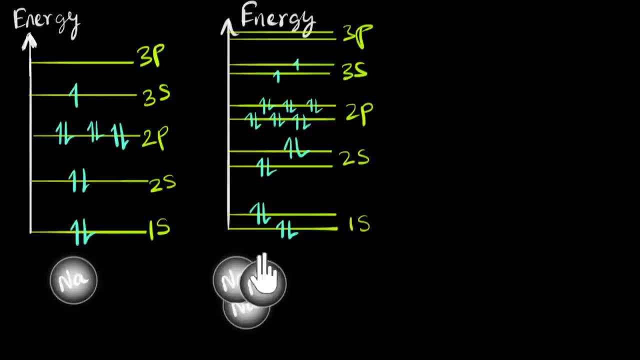 the mix. well, now three atomic orbitals are overlapping and, as a result, our molecular orbital conveniently ends up having three energy levels. three energy levels like this. i'm not gonna draw them again, so you'll end up having that. i'm gonna draw somewhere over here. now each molecular orbital will have three energy levels and i think now you can understand where. 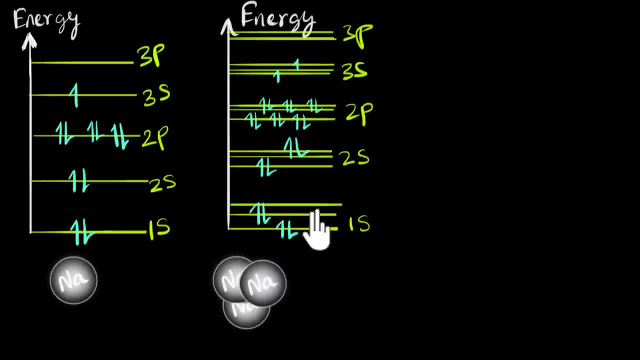 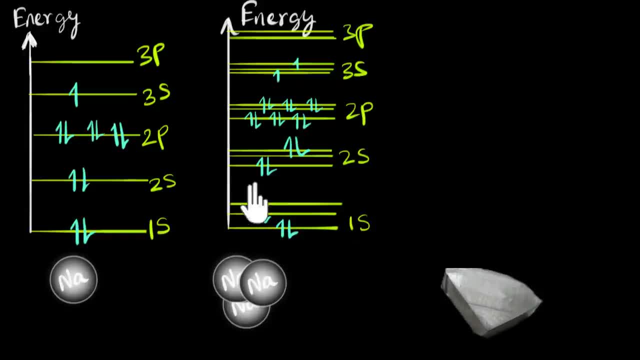 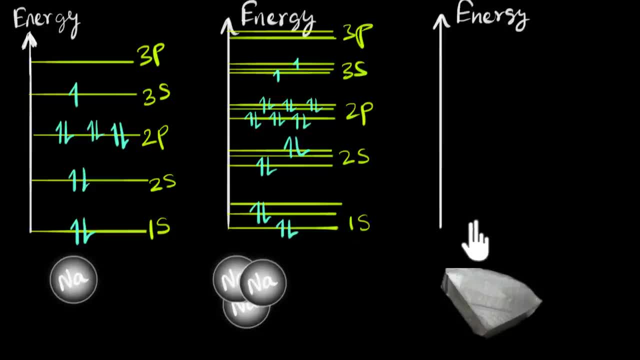 molecular Orbital of this entire solid will have now ten to the twenty three levels. so if you're a draw this, this will be interesting. what would that look like again? this now is the energy level of all the electrons of the of the solid and now the one as molecular orbital will have ten to the frei AC dar. a proposed order. 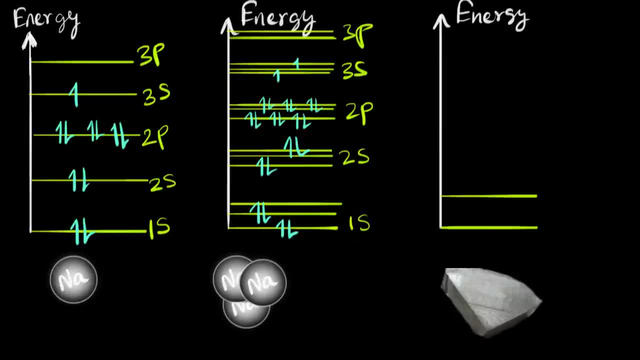 topmost one, and then all I have to do is fill 10 to the 23 levels. that's easy. Here's how I do that. I mean, think about it If I were to draw 10 to the 23 levels inside. 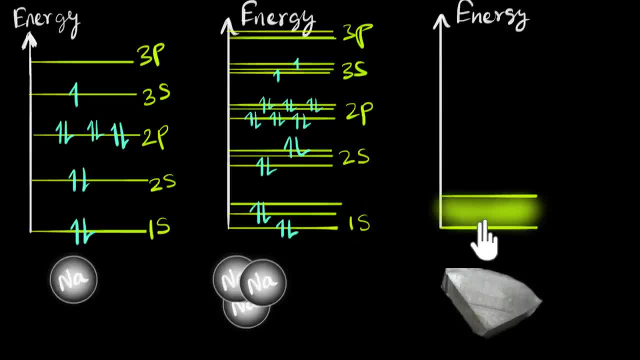 don't you think? this is what it would look like: 10 to the 23 stacked up lines. that's what it would look like, right, And so notice, no longer can we identify individual energy levels, because the gaps between them would be extremely tiny. 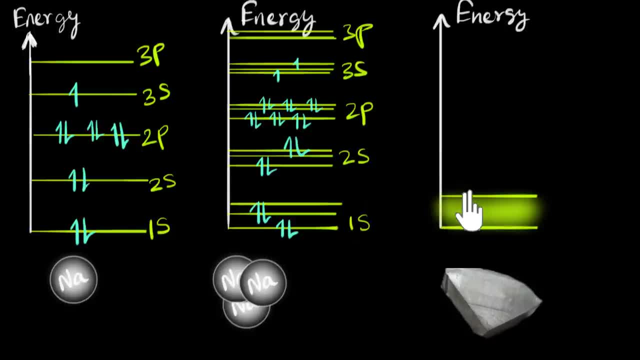 And, as a result, we like to think of this energies as continuous energies, So we like to think of this as an energy continuum. We can forget about the small gaps, that energy gaps that are present between them. And when we do think of it this way, 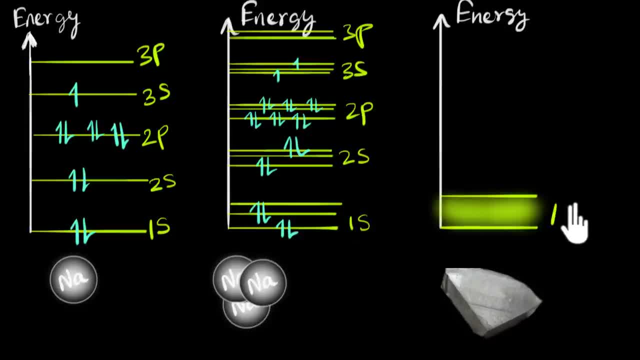 we can now call this. we can now call this as we'll not call it as a molecular orbital anymore, but instead we'll call this as an energy band. So this is called as an energy energy, energy band, Band, And the word band is signifying that we are. 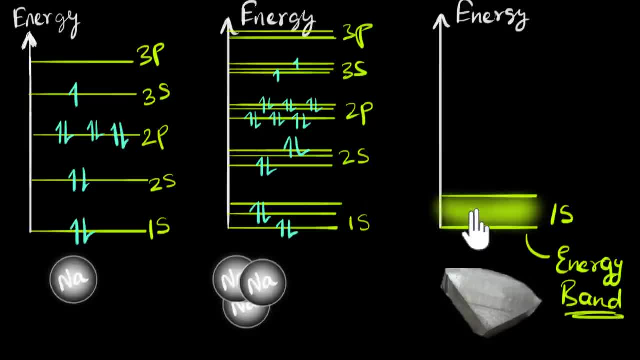 we are ignoring the small spaces that exist between those 10 to the 23 levels and we're just assuming that this whole thing is one big chunk of energy. All the energy levels, from here all the way to here, are available, continuously available. 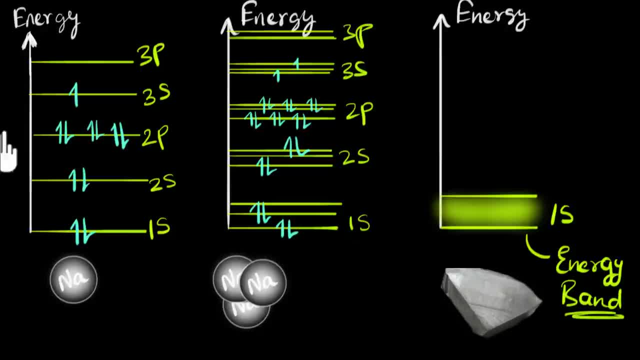 And that energy continuum is what we call as an energy band, And similarly we will have a 2S band. So we're gonna draw it the same way: I'll draw the lower one and then the higher one, and then 10 to the 23 lines in between. 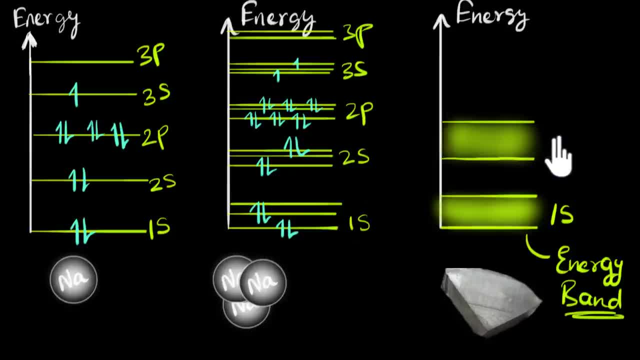 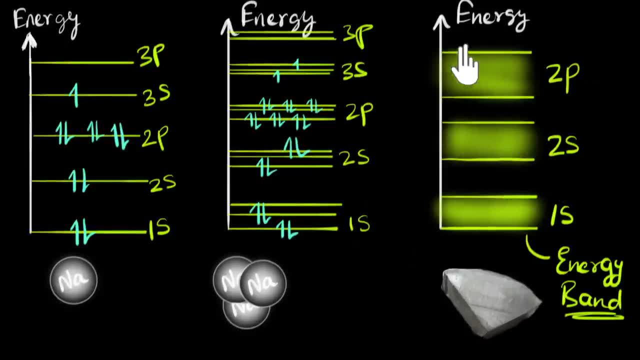 So this we will call it as the 2S band, So on and so forth. And there are other bands as well, like 3S and 3B bands. I just ran out of space over here And notice that since one single discrete level, 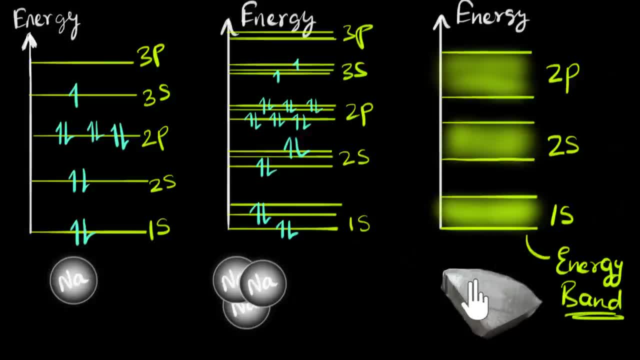 can hold two electrons. if that's the case, if there are n atoms, then there'll be n levels over here. So let's write that down: if there are n atoms over here, then there'll be n levels, and so the total number. 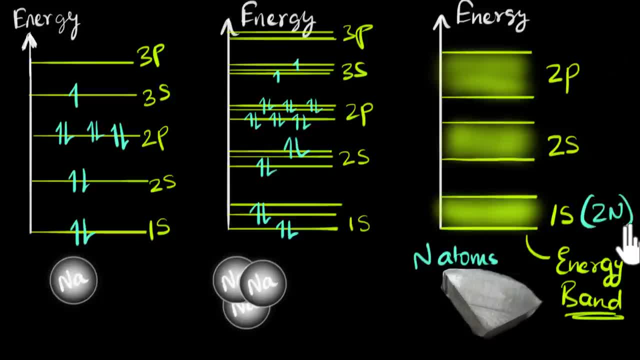 of electrons that it can fit would be 2n, So this band can fit 2n electrons. this band can also fit 2n electrons, but notice that a single P level can fit six electrons, so the 2P band can now fit 6n electrons. 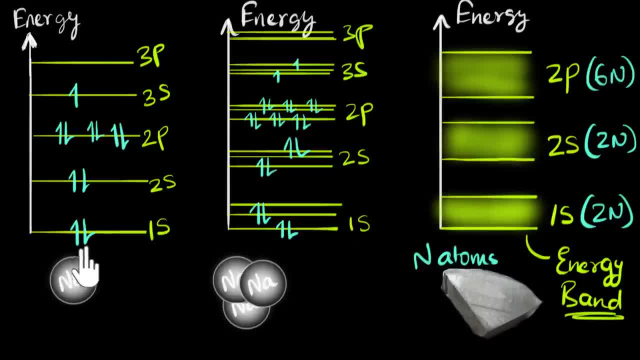 and so on and so forth. All right, to summarize: We saw that if you have a single atom or if you have a gas- Because even in a gas atoms are so far apart, We can assume they're infinitely far apart And we can pretty much assume that they're single atoms. 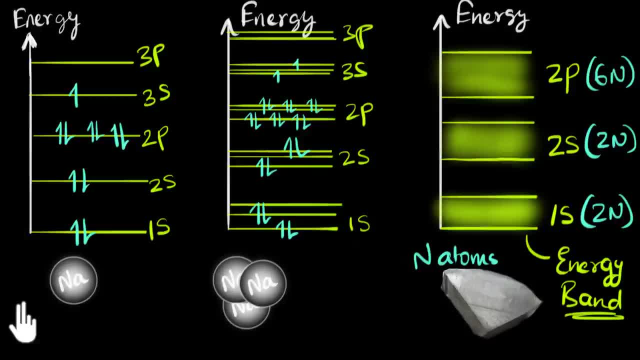 So this also works for a gas. So we can write that down: This works for a gas. So if you're dealing for gases, dealing with gases, then every electron has a discrete energy level, And if an electron wants to go from one level to another, 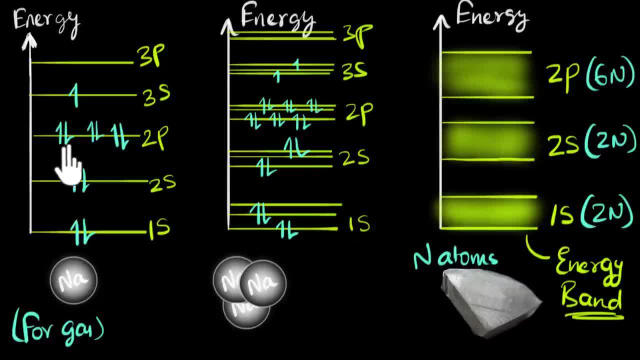 it really has to jump. There are no continuous energies available. It's sort of like steps over here. But as atoms come close to each other and eventually form a solid, they end up forming energy continuum, And we call it continuum as bands. 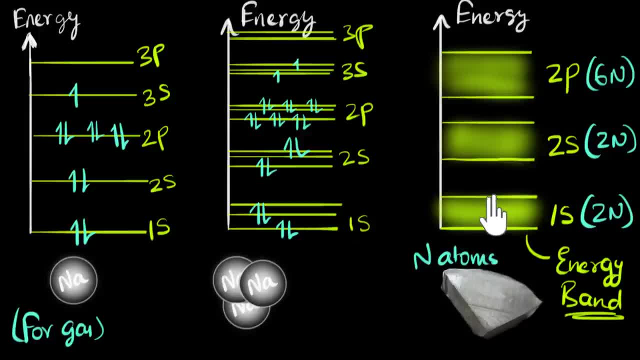 And within the bands, the energies which are available are continuous. Electrons can possess any continuous energy it wants within that band. And the name of this theory is no surprise: the band theory of solids. And now, using this theory, we can understand how free electrons are generated.